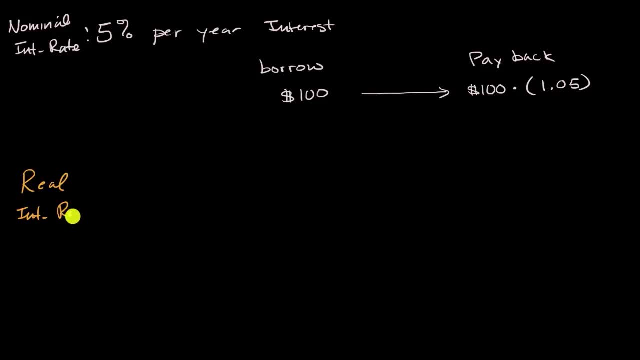 to the real interest rate. And you might say: why do we need some other type of interest rate? Well, even though on the face value I'm paying you back 5% more, that doesn't necessarily mean that you're going to be able to buy 5% more. 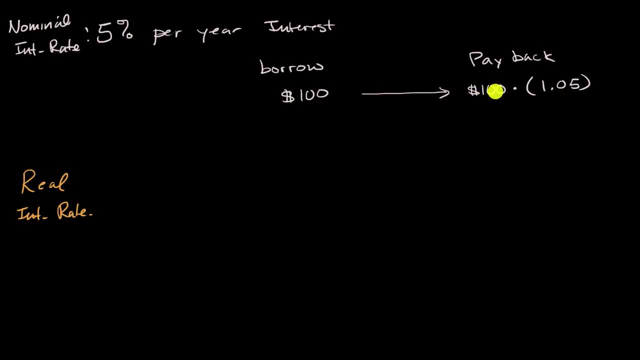 with the money that you get paid back, And you might guess why that is the case: Because of inflation, $105 will not necessarily buy you in a year what it might buy you today, And so that's what the real interest rate is trying to get. 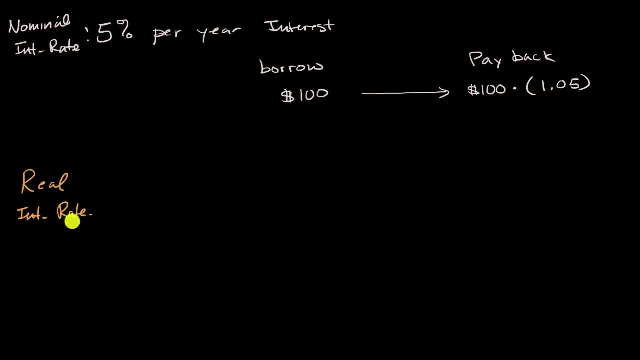 And to do that, to calculate our real interest rate, we are going to have to think about inflation. So let me put inflation right over here, And so let's say that we are in a world that has 2% inflation. So an indicative basket of goods that costs $100 today. 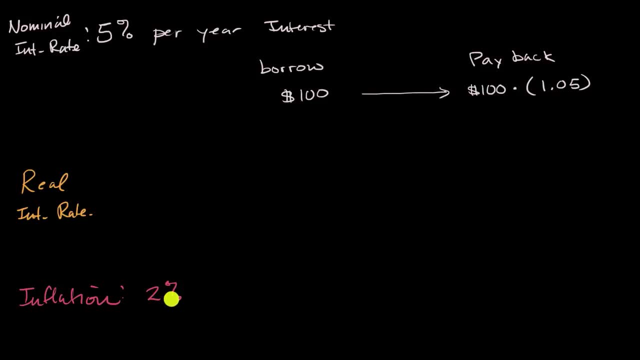 if this is the inflation rate, would cost $102 in a year. So there's two ways that folks will calculate the real interest rate, given the nominal interest rate and the inflation rate. The first way is an approximation, but it's very simple and you can do it in your head. 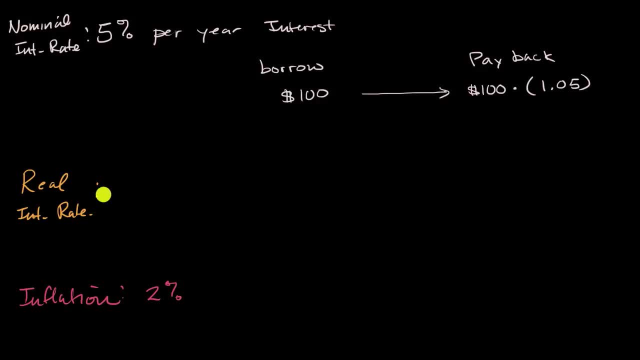 And that's why it's often the first way that it's taught. but it's not exactly mathematically correct. So the first way you'd say: well, this could approximately be equal to the nominal interest rate minus the inflation rate. So you could say this could be approximately equal to 5%. 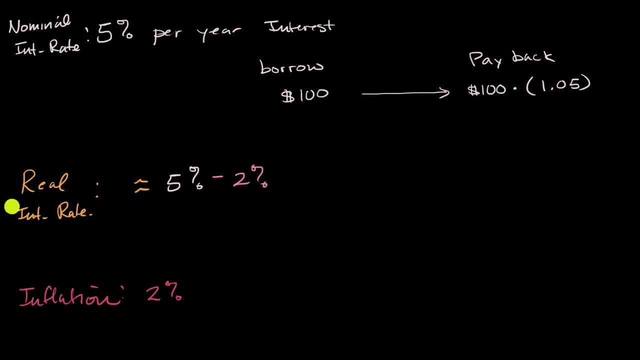 minus minus 2%, which would be equal to 3%, And this is a decent approximation. But the actual way that you would want to calculate this, if you wanted to be more mathematically precise, is that your nominal interest rate multiplies things by 1.05.. 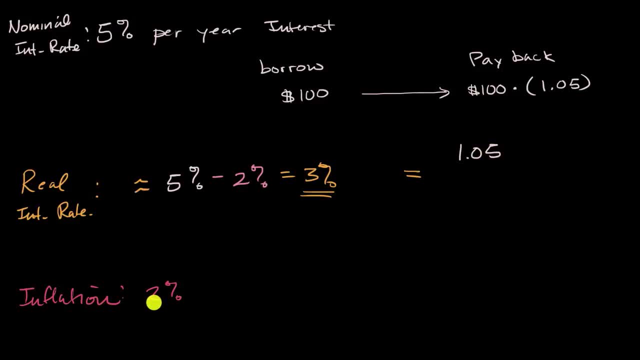 So 1.05.. But then things are getting more expensive at a rate of 2% per year, Or another way to think about it, costs are being multiplied by 1.02 every year. So we divide by that amount 1.2 every year. 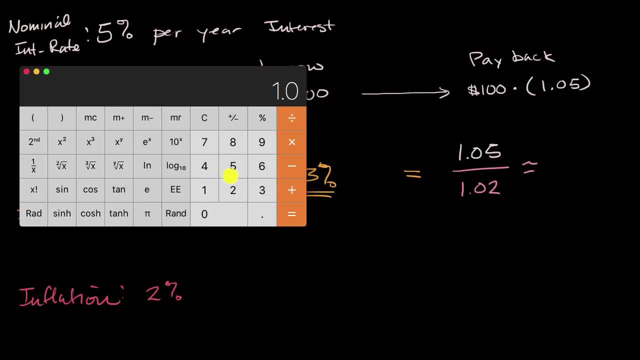 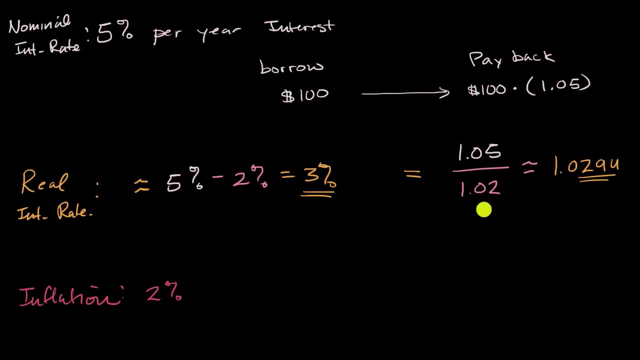 And so this was going to give us 1.05.. Divided by 1.02 is equal to 1.0294, 1.0294.. And another way to think about it, we just got a much better sense of what the real interest rate is.